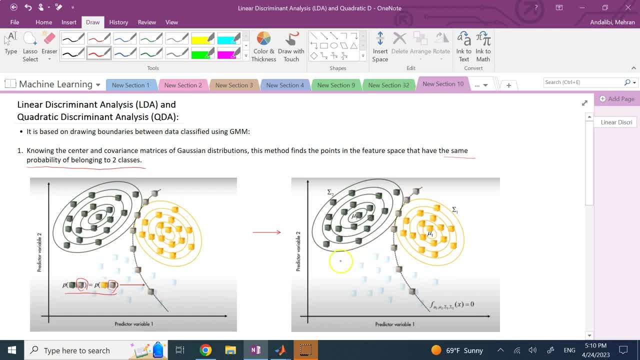 of them, f1 of mu1 and sigma1, and the other one f2 of mu2 and sigma2, and then I say these two are equal and then take both of them to one side. so f1 minus f2 is equal to zero, and I call that f1. 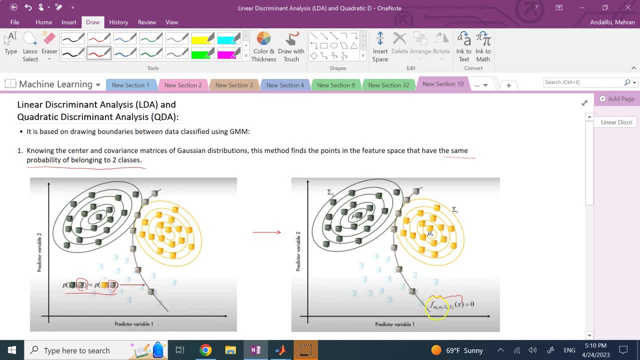 minus f2, the f in general of this four parameters at x equals zero. then I can say: this is the relation that you need for what? for the classification boundary. so this one and this one are what. these are equivalent to each other, whether you describe it by equality of these two conditional probabilities or you say: 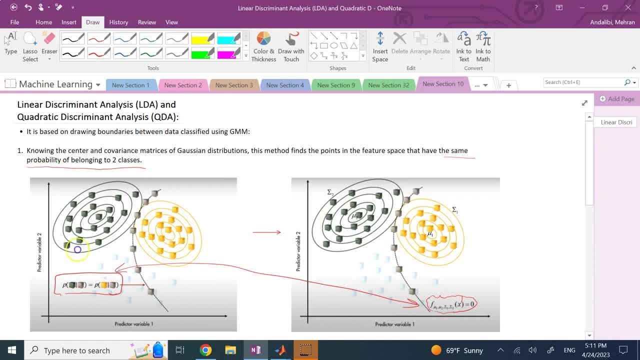 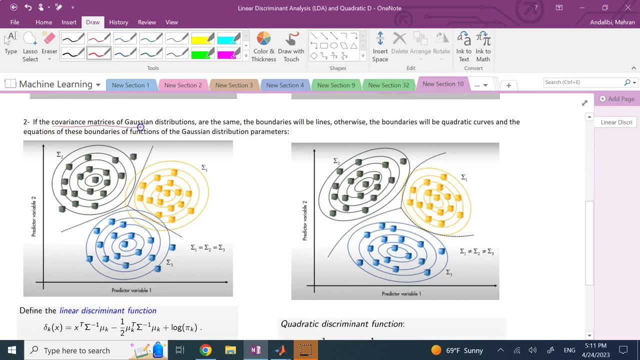 this way. that's basically the same thing. okay, so the goal is to come up with the boundaries. now, if the covariance matrices of these clusters are the same, then you can easily show that what the boundaries will definitely be lines. okay, so the boundaries will be lines. mathematically, you can. 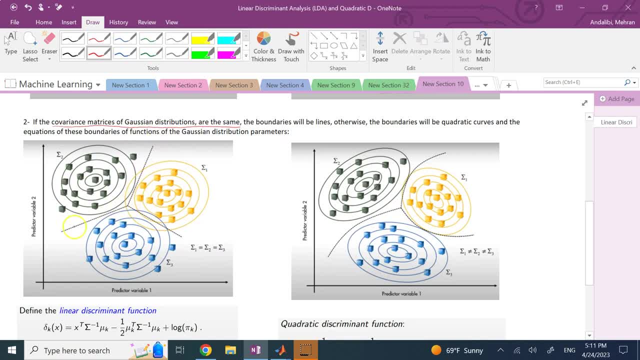 show that the when you connect these points together, with equal probabilities they would be on a line if the sigma one, two, three are equal. on the other hand, if they are not equal to each other, then the boundaries will be quadratic. curves will be like: x2 is a quadratic function of x1, and so this one on the left, we call it linear. 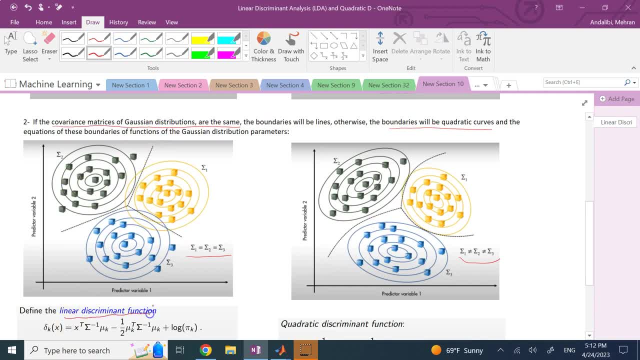 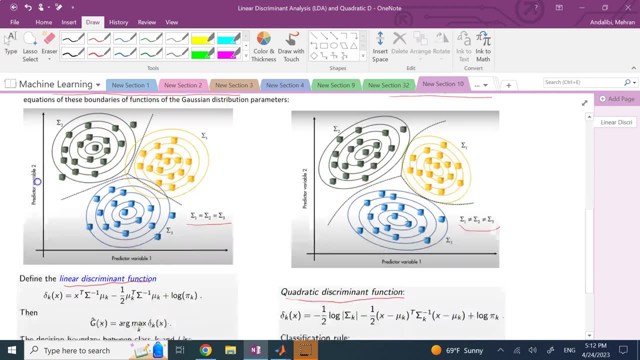 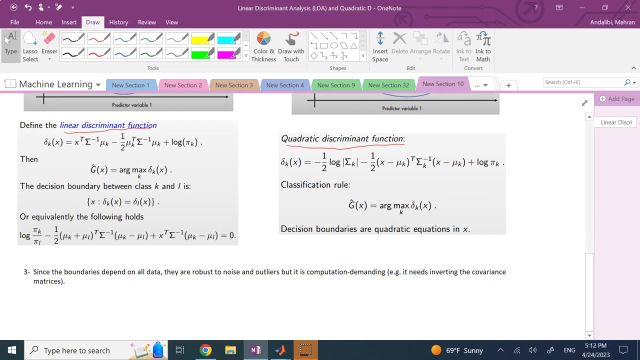 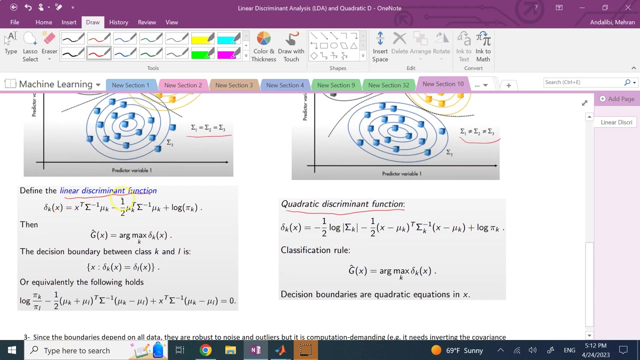 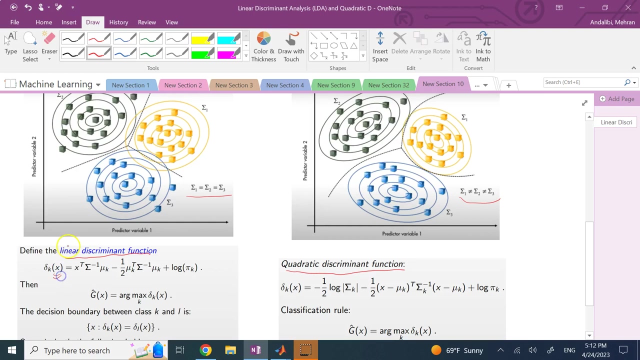 discriminant function or linear boundaries. the one on the right, we call it quadratic discriminant function or analysis. and this guy is called lda, this one is called qda. okay, now, what are the forms of the bases? so the constraint distribution statement is the constant equation of poured Jane right. the expression of codes is the vibration of the. 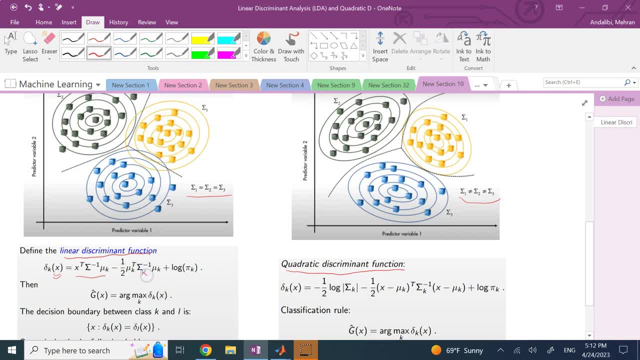 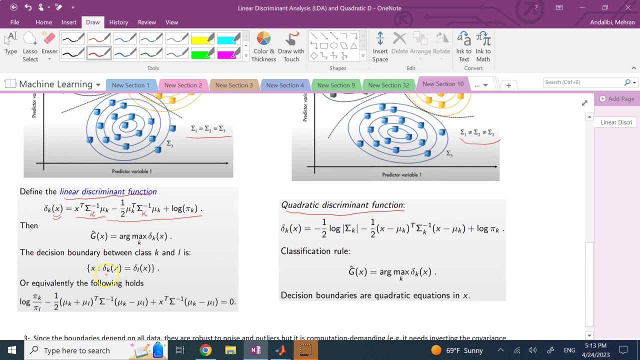 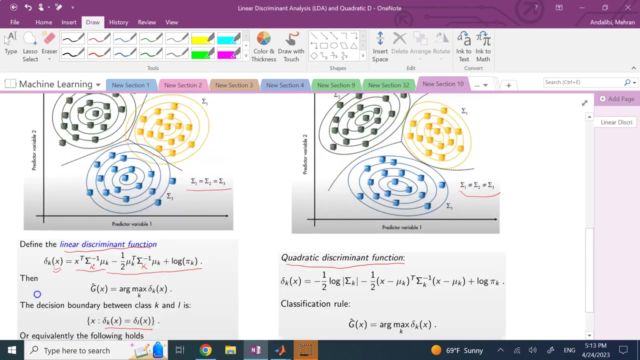 sigma, by the way, is sigma of k. okay, so this is also sigma of what that's, the cluster k. so this is what this is: the linear discriminant function for uh, one cluster, and if i set it equal to the linear discriminant function for another cluster, if these two delta functions are equal, that is. 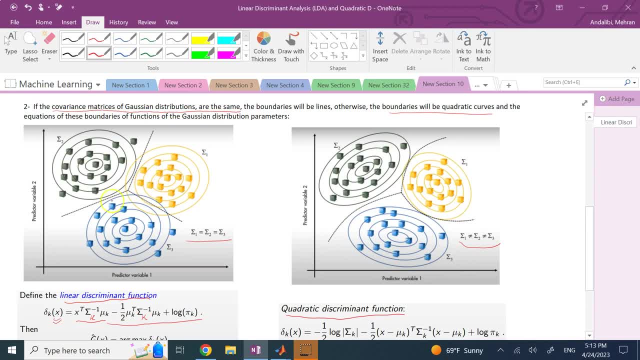 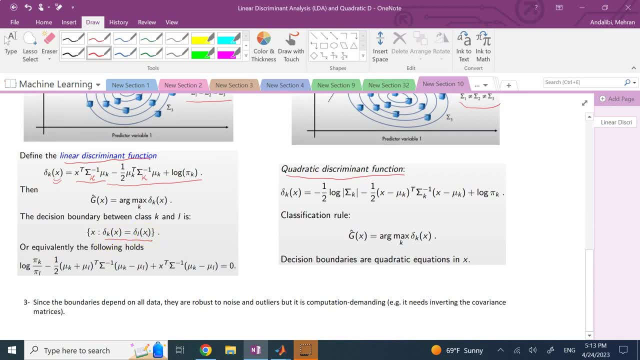 where these probabilities are equal and that is where the um boundary lies, right. so all of the x points for which these two deltas are equal, those are the boundary points, and if we set them equal and bring everything to one side, then clearly the equation of the boundary is going to be this guy. 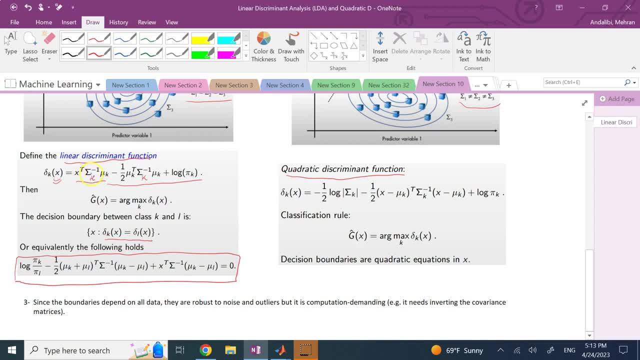 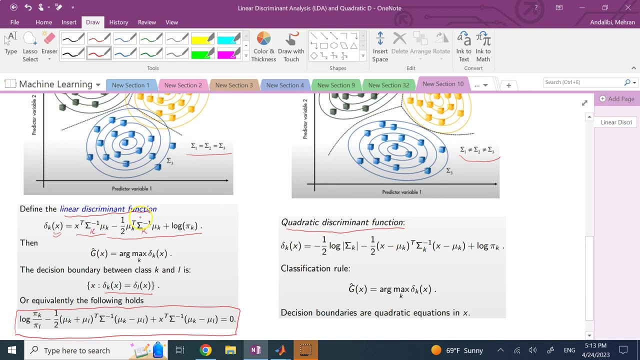 here right, you can see that this x transpose sigma inverse. is there mu k minus mu l. now you know that there is a mu k and a mu l, but they are what they are, equal. that's why here we did not use a subscript for sigma y, because sigma of l and sigma of what k are the same thing, so they are all equal. 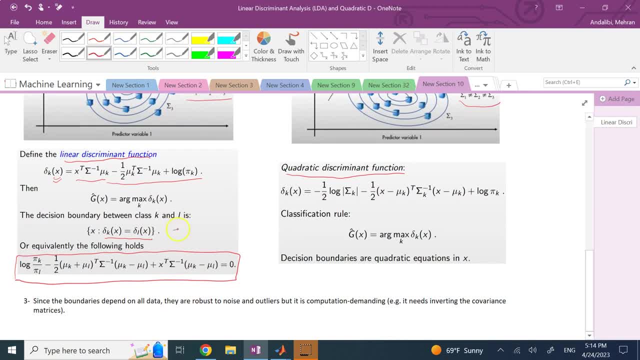 to sigma, right? that's why we only use one sigma and not several sigmas. so we factor it out and then this one half term mu, the mus are different, so you have to factor it out like this, and then these two logs when you subtract them, it's going to be. 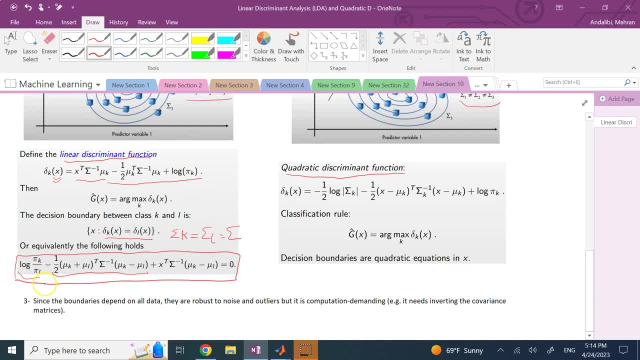 the log of the division. and if you look here, everything is a number except for x, right? because, uh, the pi k and pi l are known numbers, so this is a single number here. this is a single number, this is a single number, this is a matrix, so this whole thing will be a number. and then here, uh, this is. 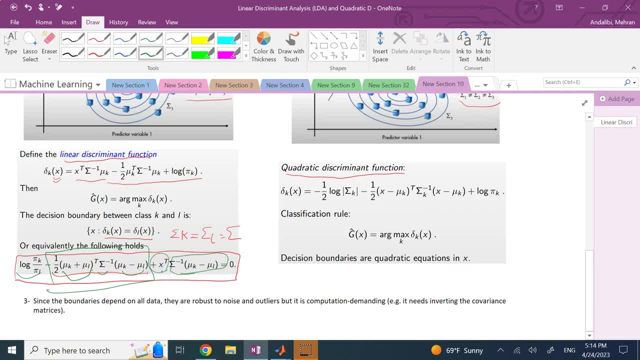 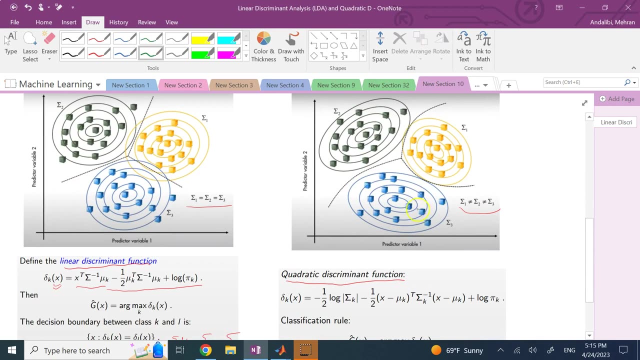 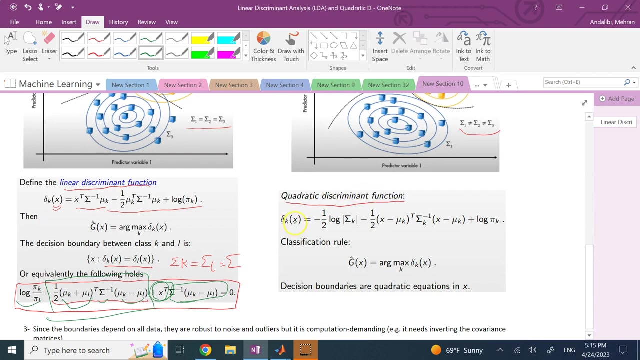 also a, a number or vector, multiplied by x transpose. so, in general, the only term of x that you see here is, this guy, a linear term of x. so, clearly, the boundary is going to be what is going to be a line, as you can see. on the other hand, if, uh, the sigmas are not equal, then your quadratic discriminant function is this: 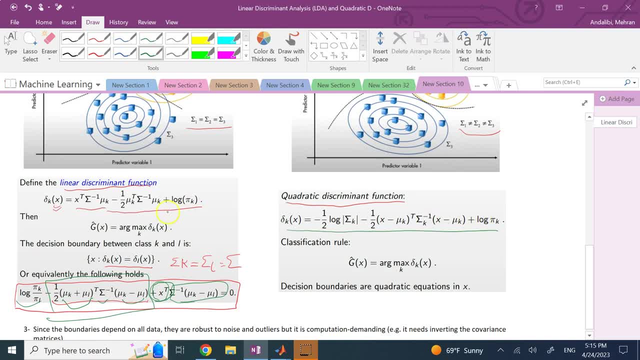 function here and if you look at it it's quite a bit similar to the uh linear one, with some differences. what is the difference? the log pi k is there right. here you have a constant term negative one half log of Sigma K, right, which is in place of. 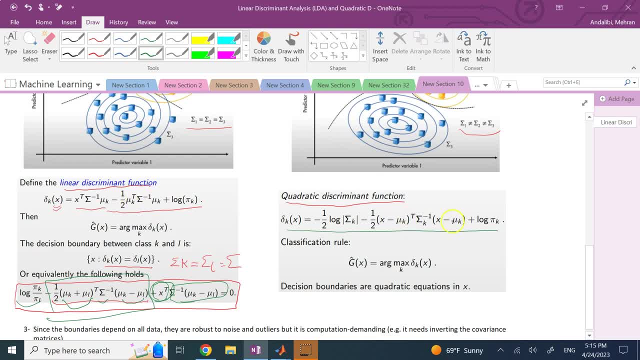 this constant term here and then here you have a quadratic term in terms of x again. if Delta X is the same as Delta K of X, is the same as Delta L of X, then that gives you what? that gives you a quadratic curve, and the reason for that is you have a quadratic function equal to another quadratic. 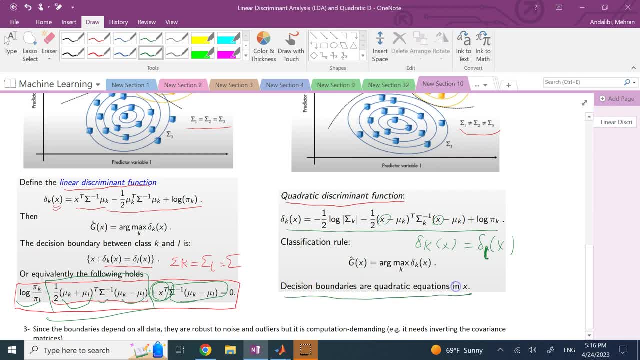 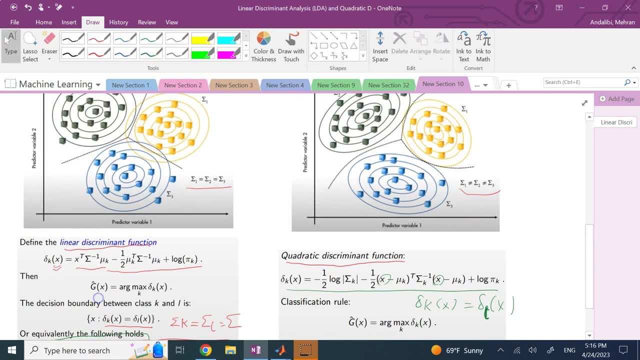 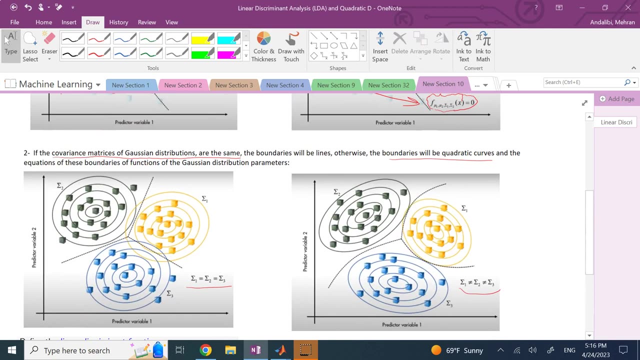 function right, and so the decision boundaries can be what quadratic? you can simplify this in terms of quadratic terms and linear terms, but in general, it's going to be what it's going to be: a part of a parabola. so this is what this is: linear and quadratic discriminant. now one other thing before we go. 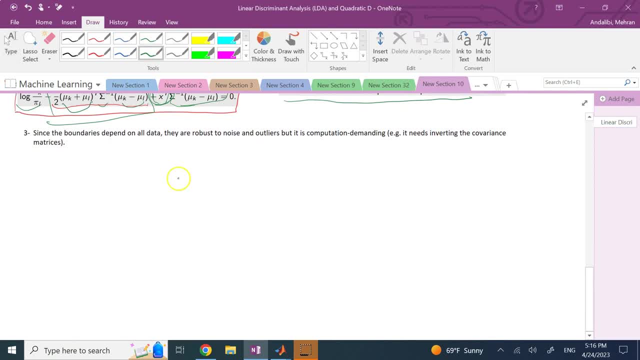 to the math lab code and the fact that the boundaries they do depend on all of the data, right, remember, in support vector machines our boundaries depend only on what? only on the support vectors, nothing else. so that makes the computation a little bit less intensive. here the boundaries: 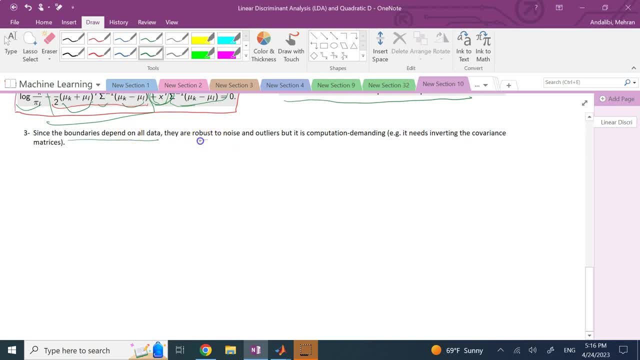 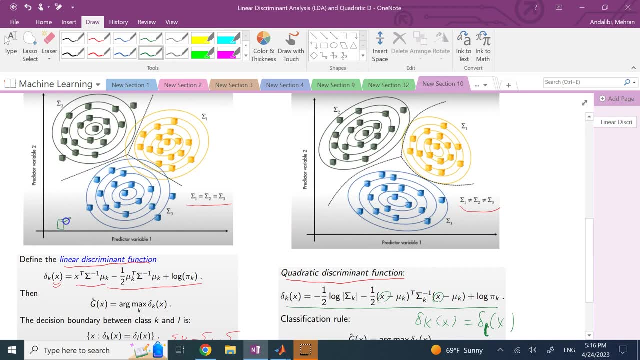 depend on all of the data. that's why they are robust to noise and outliers. so if you add an outlier, blue data here- right, it's not going to shift this boundary and this boundary really significantly. or if you add some noise, because all of the data will determine the boundary and not one, and you might say: where is it that all of the 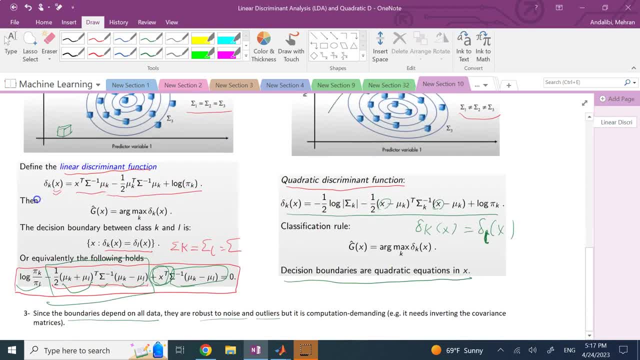 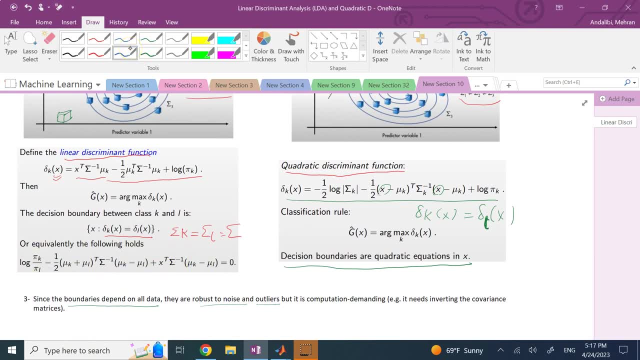 boundary is determining all of the or the boundary here, because this is the equation of the boundary right, this is the equation of the boundary here. so where is it that all the data is showing? because, as you can see here, uh, the parameters that are affecting the equation of the line are what? Sigma, mu K and mu L. these three parameters, 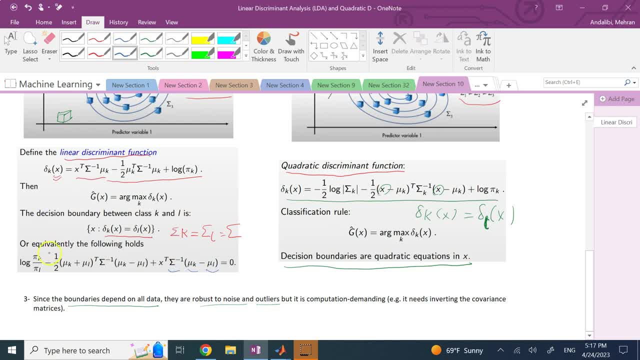 that's all it is, and these constants pi K and pi L. so where is it that all the data is coming up? and that's exactly where you calculate this Muse, Sigma and pies. you know they come from what they come from- all of your data. just in my previous lecture, when I talked about Gaussian mixture models, I showed you that when 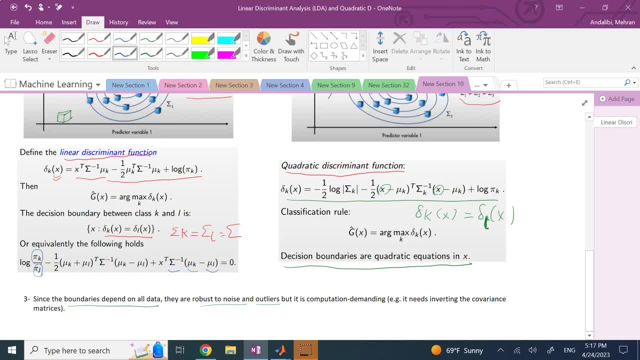 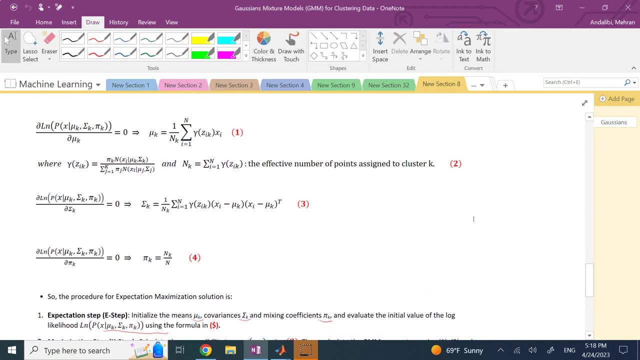 you want to calculate mu, Sigma's and pies, you have to use all of your data right. so if you go and look at these formulas in my previous lecture, you can see that I need to use what I need to use. go over each and every one of my observations: right for mu, for Sigma, right, I have to go over all of my. 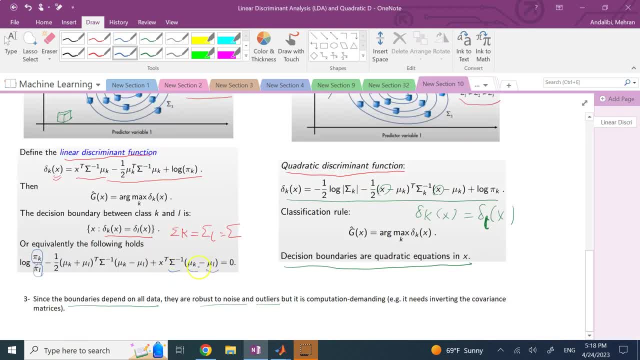 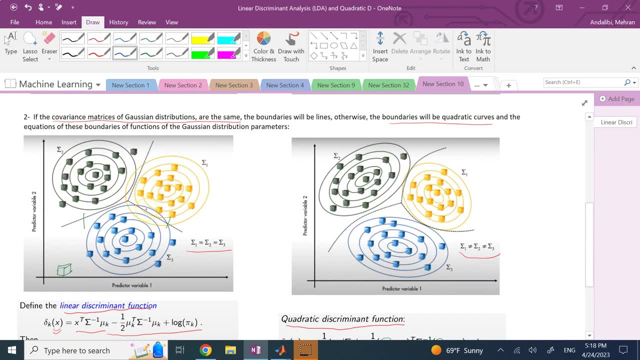 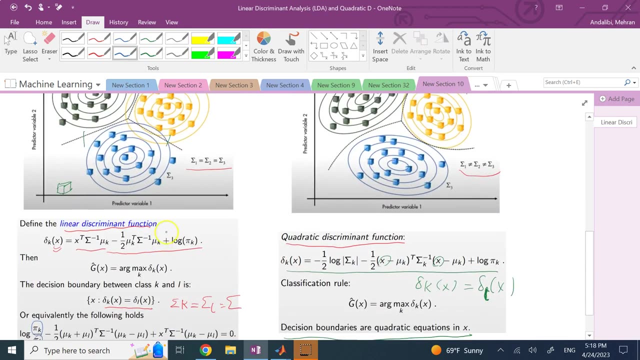 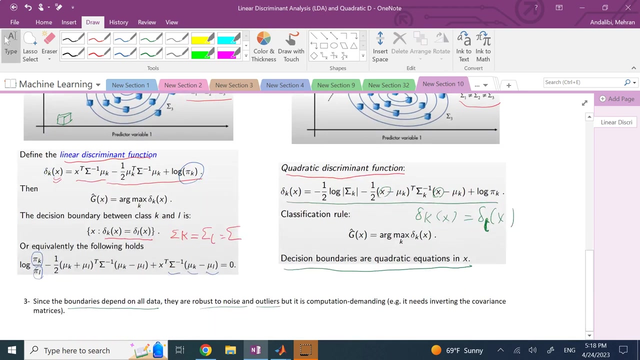 observations. and that's why, uh, when you pass your data X, your X data observations and the labels to the uh discriminant function in math lab, let's say, it has to first determine the Muse, Sigma's and pies. so first it has to perform a GMM, then it can find the boundaries for you, okay, and it is therefore a. 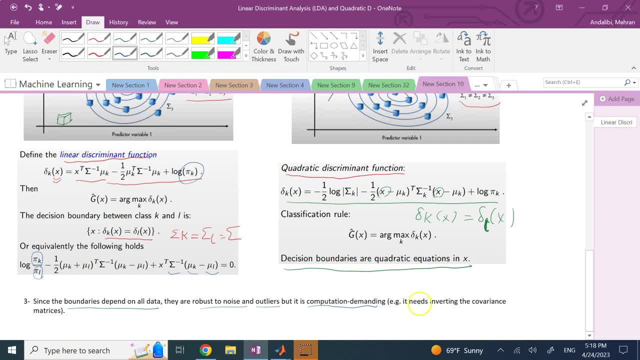 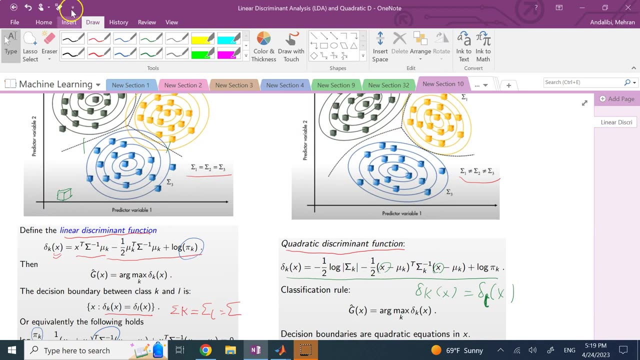 little bit computationally demanding. okay, and the other thing for demanding the computation is it needs to invert the covariance matrices as well, which you can see here. and for this case where the the matrices are two by two, it's not a big deal. but when the dimension of the feature space is very large, inverting that big. 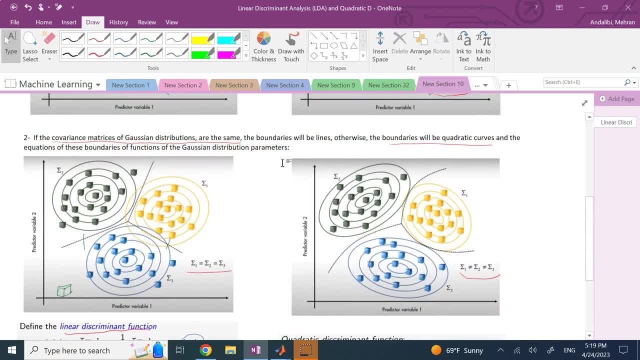 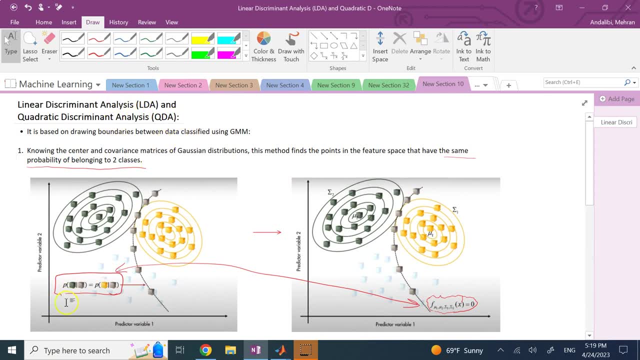 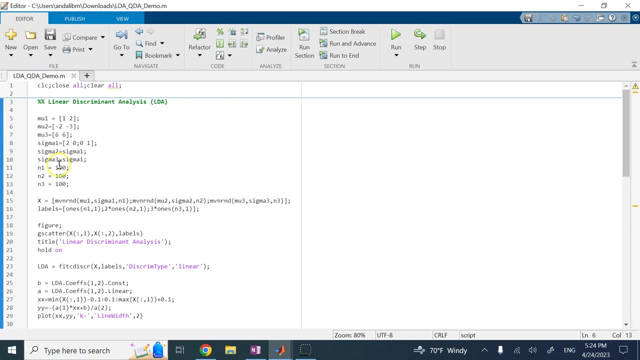 Matrix also could be computationally demanding. okay, but uh, this is in general what the simple theory of LDA and QD a. now let's take a look at some math lab code together. okay, so here is the math lab code and, uh, here I have three Muse, three Sigma's and three ends for LDA. I use my Sigma two and three to be. 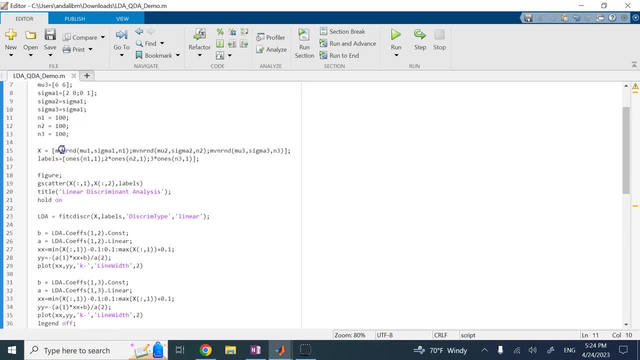 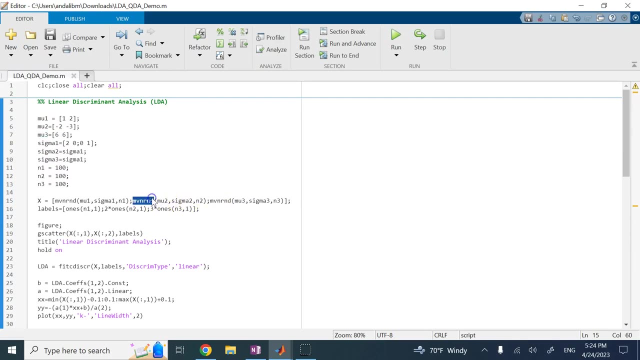 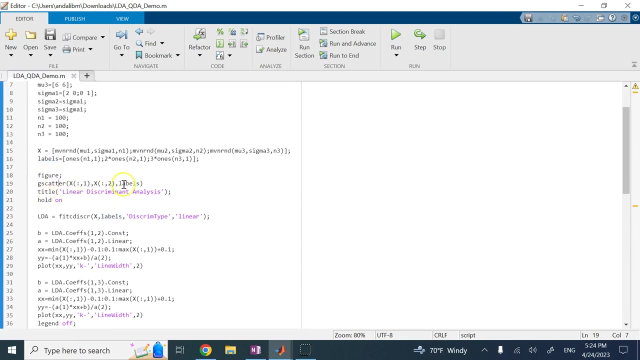 similar to the same as Sigma one and uh. I use my MVN rant command to generate random numbers from the multi-variable normal distribution and, using a mu1, Sigma one and one and similarly for two and three, concatenate them together, create the labels for them and use gscatter to do the scatter plot with different colors for different clusters. then I use 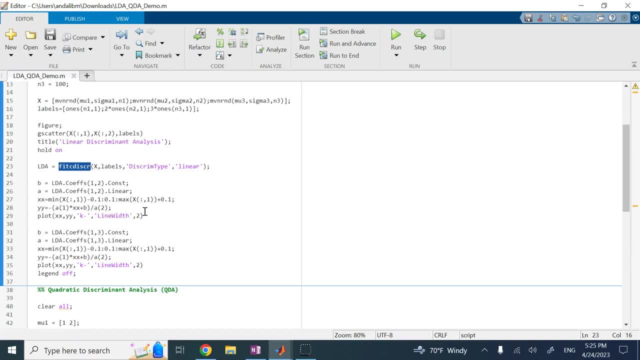 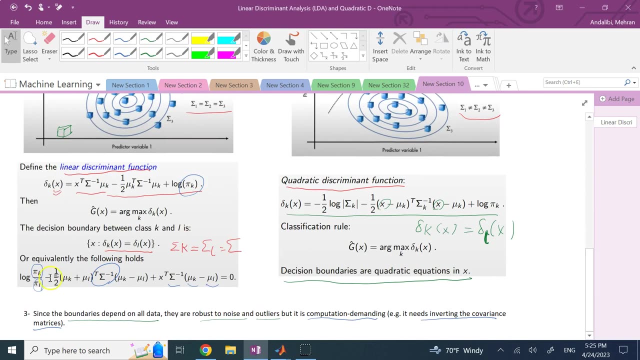 the command fit C. this CR and fit C discriminant is. I pass to it my training data and the labels, right? so you see, I do not pass to it any mu or any Sigma or anything okay, which you need for the equation of this line. so the algorithm has to. 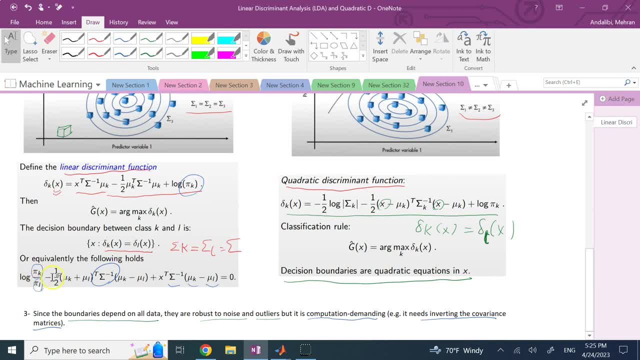 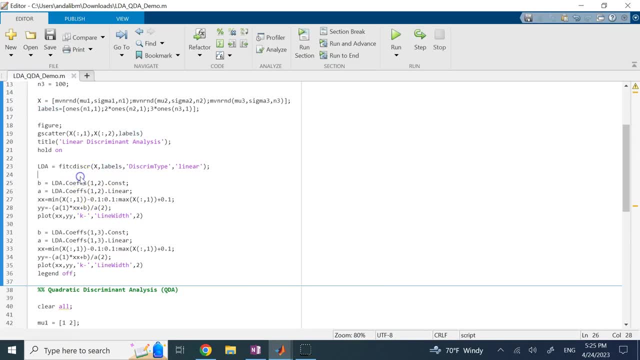 find mu, Sigma and the pies first, then find the equation of the line right, and that takes some computation, so it calculates that and then, since it's linear, I get the coefficients out of this LDA, and first I do it for between class one and two right, and I get the constant out of it. 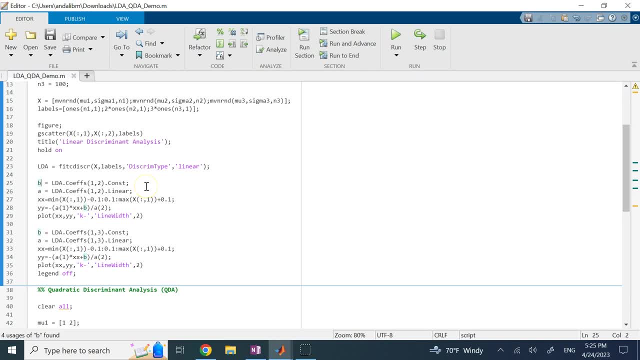 so it's a linear coefficient right and the equation of the line is going to be: a times X plus B equals zero. but your X has two components, x1 and x2. so your equation is going to be what is going to be basically a number one times x1 plus a number two times x2 plus B equals zero. 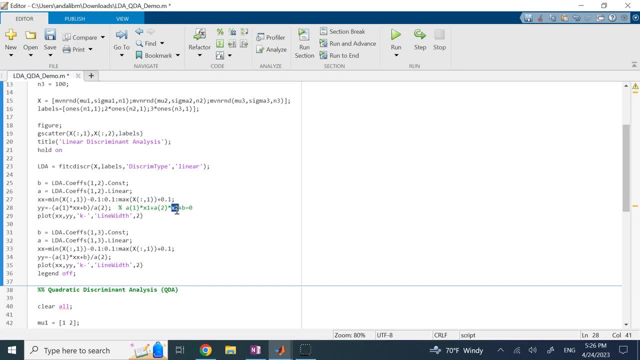 okay, here x1 acts like x and x2 acts like y. basically that's the equation of the line. and now if i form my x1 through some column operator here, from the min of the x minus 0.1 to the max of the x plus 0.1, with increment of 0.1. 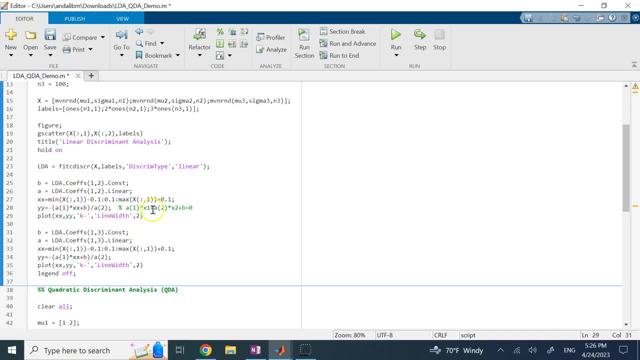 and then my x2 or y. i get it from this equation: i take a1, x1 and b to the other side and divide both sides by a coefficient 2. that gives me the x2 or yy in this case, and then i plot my xa and. 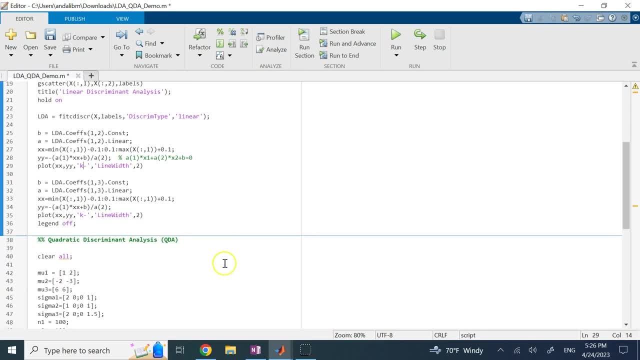 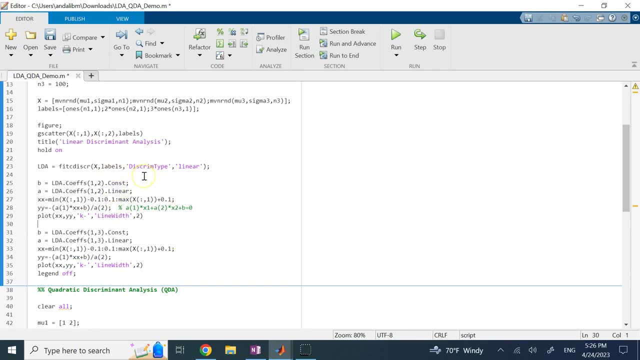 yy with black color to form the line. and then i repeat the same thing, this one between class one and three instead of class one and two, and here one and three are basically. one is in the center, here two and three are on the sides. so i do one, two and one three and i get my two. 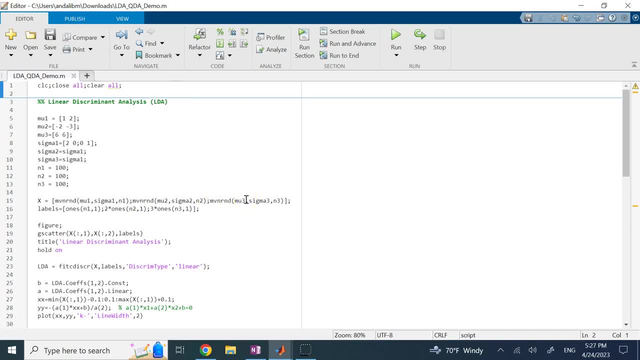 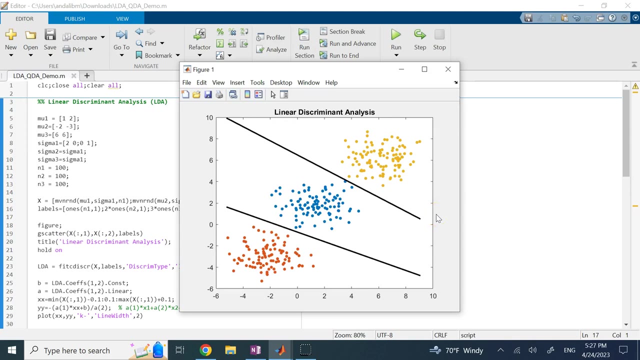 classes. now, in general you can have three lines. you can do one also for two and three, but in this case i really don't need that, so i just do one and because the way the classes are separated, two of the lines are enough, but in general you can generate three lines. okay, so this is what you got. 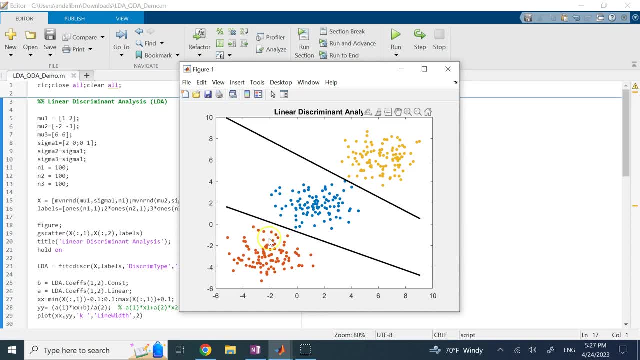 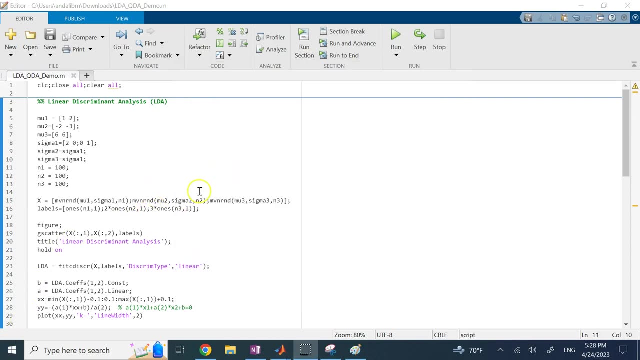 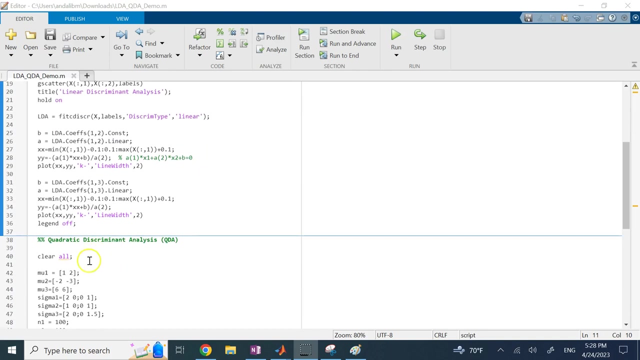 this is one class, this is one class and this is what one class and these are what. these are the lines separating the classes of data together. so this is what. this is my linear discriminant analysis result. then i go ahead and i create um the qda, so this time i create new set of data. i. 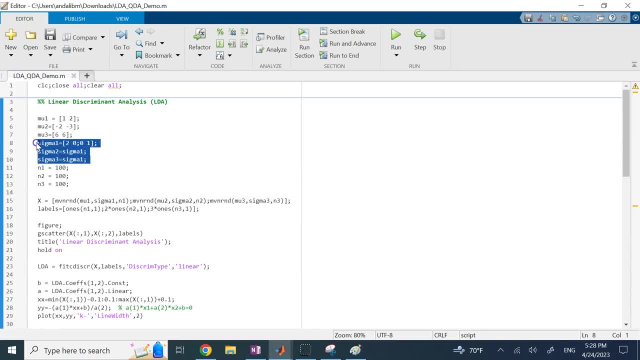 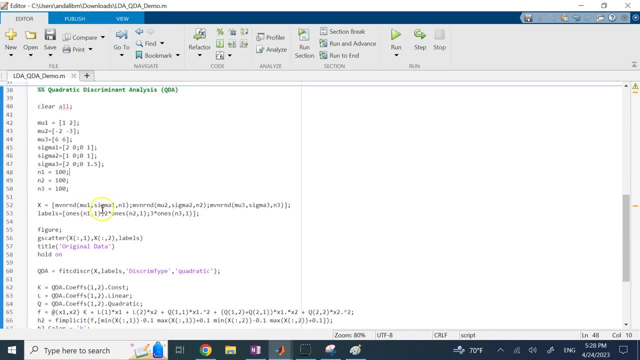 don't need to do it on the original data, and the reason is i want my sigmas to be different this time. so here i use different sigmas matrices and again i generate my data label and everything, and this time the only thing i change in this fit c: discriminant. 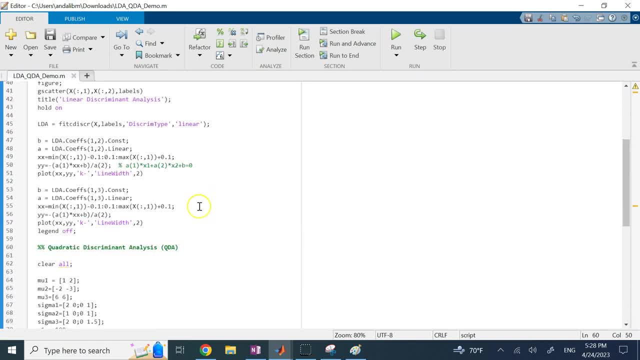 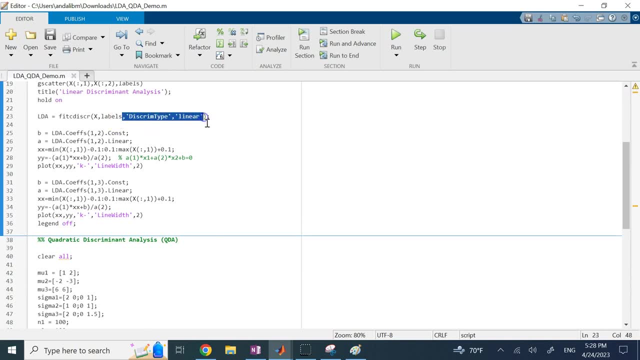 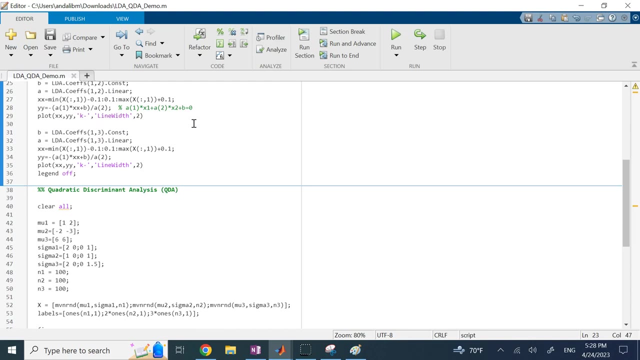 is the discriminant type and i pass it quadratic. last time it was what it was- linear. and since it's the default, if you just eliminate this part of the code altogether and again it's going to give you linear. so if you don't say discriminant type, it assumes it's linear. but you can say it if you. 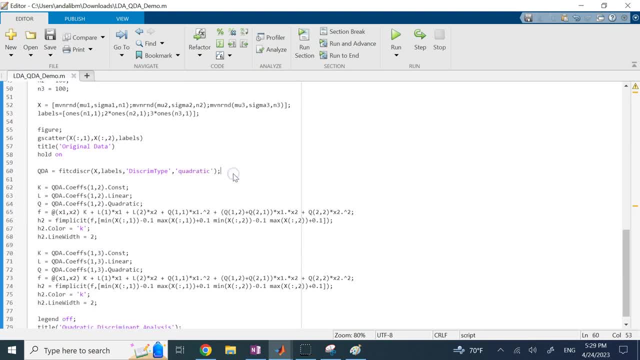 want, and here you have to definitely say that it's quadratic. so you generate that now. this time the equation of the line is a parabola. so if i go between classes one and two, you have three coefficients: a constant, a linear term and a quadratic term, and i call them k, l and q. 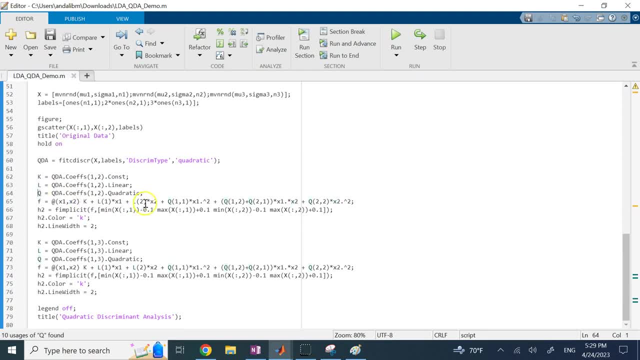 and the thing is, the l and the q are going to be multiplied by what? by both x1 and x2. so you see here, the components of l are multiplied by them and the component of the q are multiplied by them. so, if you have x1, in order to find 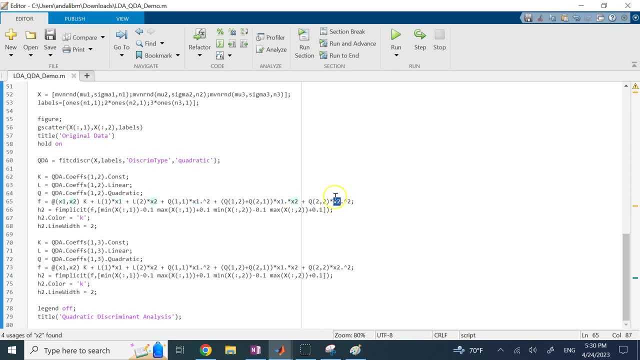 x2. you have to use a. what you have to use a quadratic equation to solve for x2. that's one way to do it to find it explicitly: x2 in terms of x1. so you have an equation like that right. or you can use an implicit function here in this case. so here i create an anonymous function. 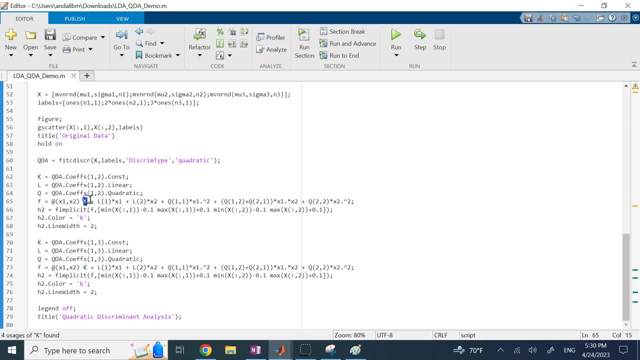 of x1 and x2, which is the constant k plus l1 times x1 plus l, number two times x2, q11 times x1 squared plus q12 plus q21 times x1 times x2 plus q22 times x2 squared right. that's the equation. 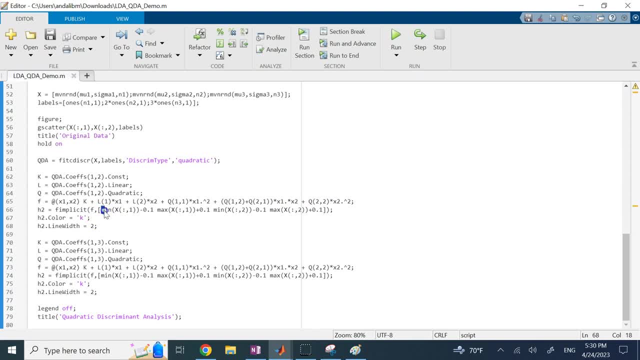 quadratic and what i do. i'll pass the whole range of my x and y, or x1 and x2 in this case, and the function to something called f implicit. okay, and you might say: what is this function? f implicit, because i passed to it as an argument the handle to an anonymous, anonymous function and some x mean x max. 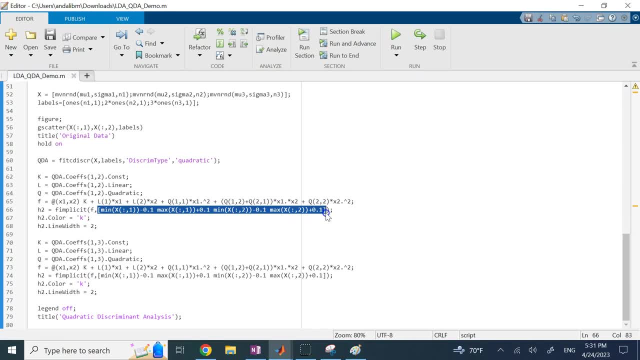 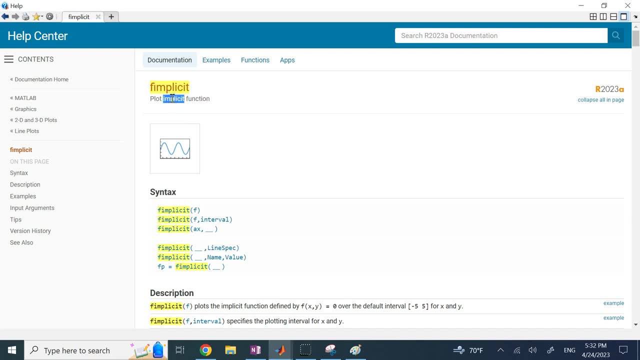 y min, y max, or x1- x2 min and x1- x2 max. so here is the math lab help for it, and this is a beautiful function which plots implicit functions, so you don't have to find x2 from as a function of x1. 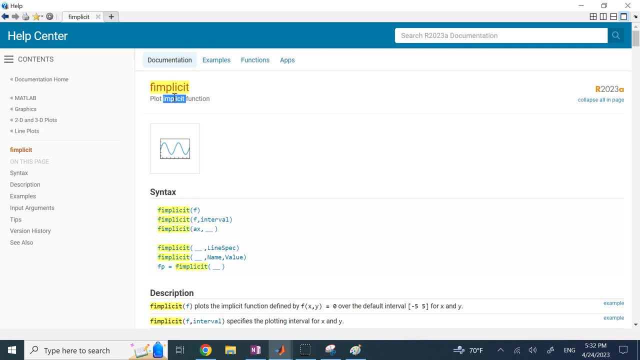 an implicit function and then plot it. this guy, if you give it a relation, an implicit relation between x and y and x2, you get the function. that's the function. that's the function that's x and y, without the need to solve one based on the other. it plots it for you all you need to pass to. 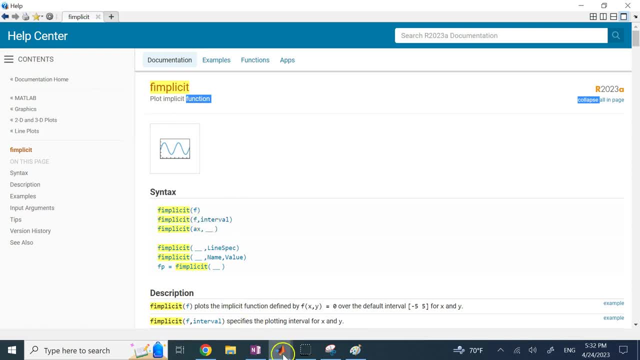 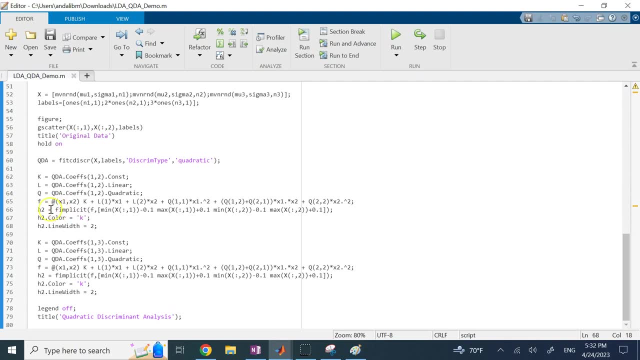 it is the function and the interval, as you can see. so that's a beautiful function which i can use here, and for color of it i pass k, for line width i pass two, and you see here that plot has a handle, so i can modify its properties using the dot operator. okay, so now i plot my um first parabola.